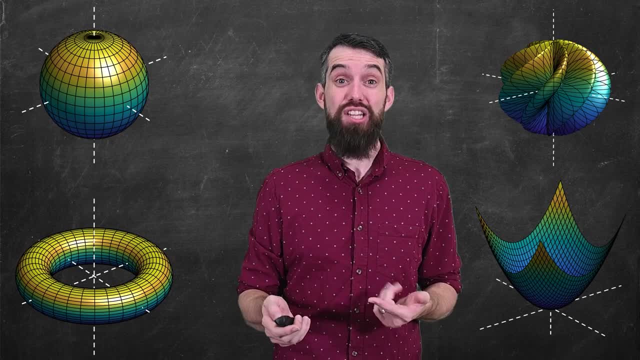 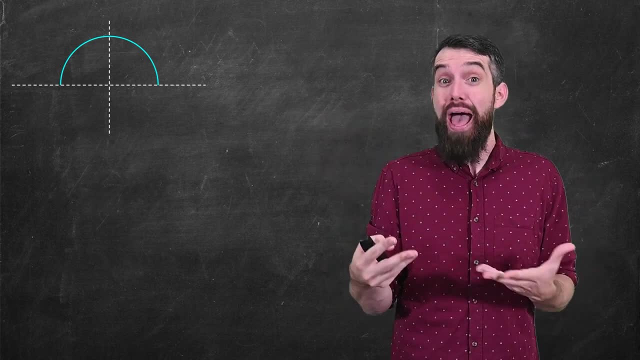 we mean by that in a little bit. Now, the first thing I want to do is actually go back to the study of curves we've done before, because we've seen that for a curve like this- the top half of the unit circle- that there's actually three ways that we can describe this. 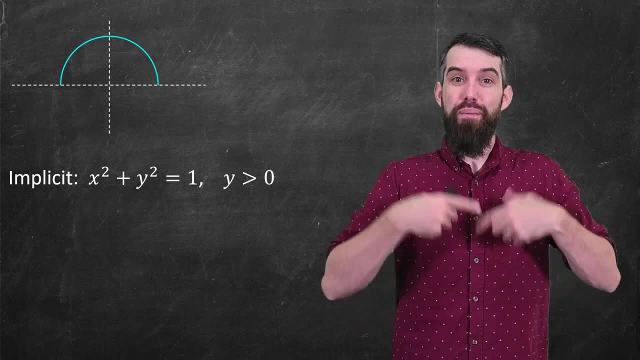 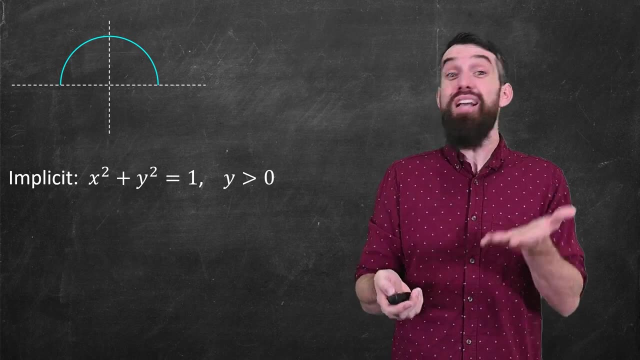 We can describe this implicitly. So this is when I just give some function of x and y and set it to be a constant. In this case, x squared plus y squared is equal to one. I could solve it explicitly, which is when I take my formula and I try to solve it for. 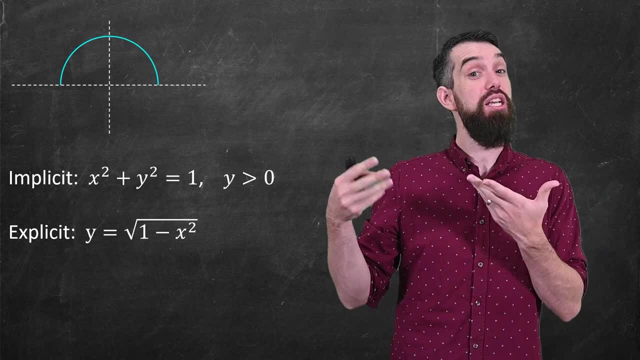 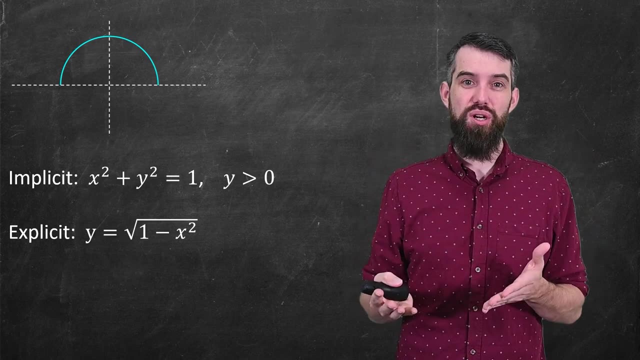 one of the variables, like y, is some function of x, In this case square root of one minus x squared, And I chose specifically that we were only doing the top half of the unit circle because then I can solve it and I don't have any weird plus or minus issues coming up. 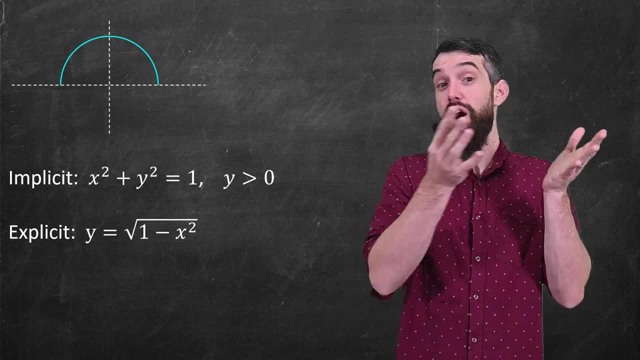 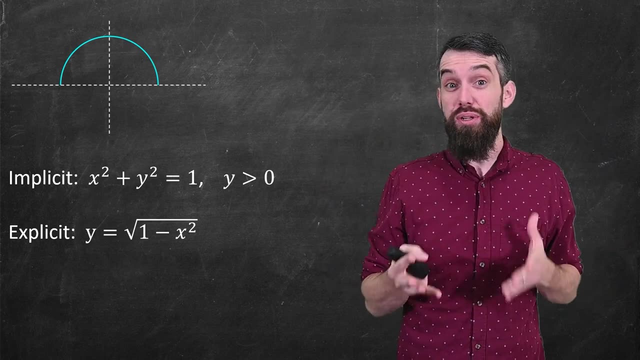 In general, though, it's often not possible to start with an implicit formula and to generate just a single explicit formula for it that works for everything. This, in general, is not possible, So it's only sometimes that I would have an explicit formula for my curve And then the 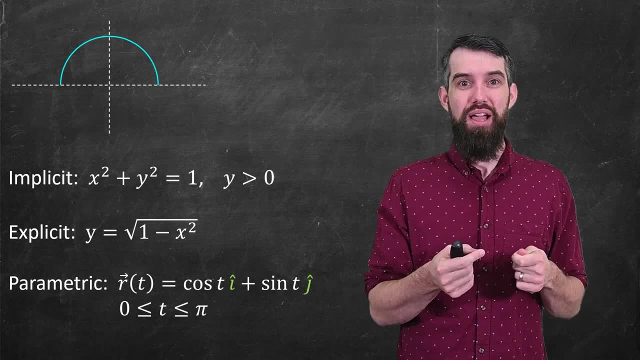 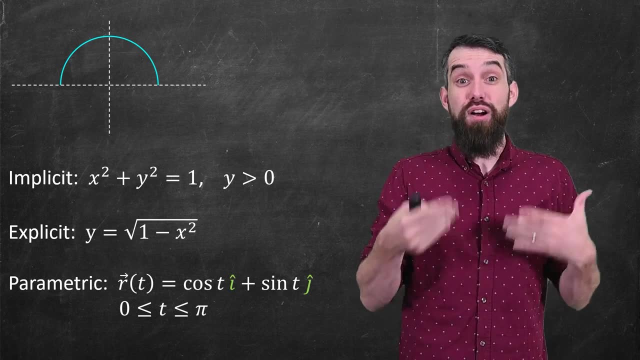 third, and the one that's going to be most important for us, was the parametric form. This is where I take some parameter or t and then I specify some function in the i-hat- in this case it's cosine of t- some function in the j-hat. 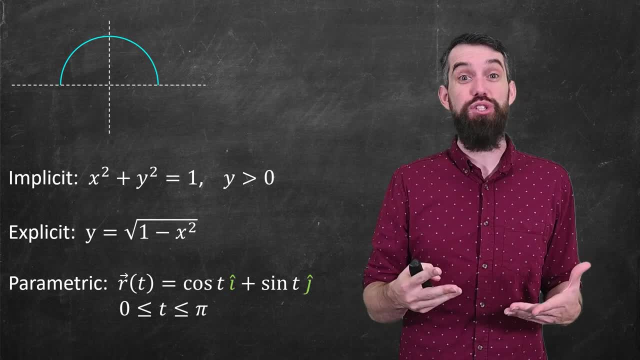 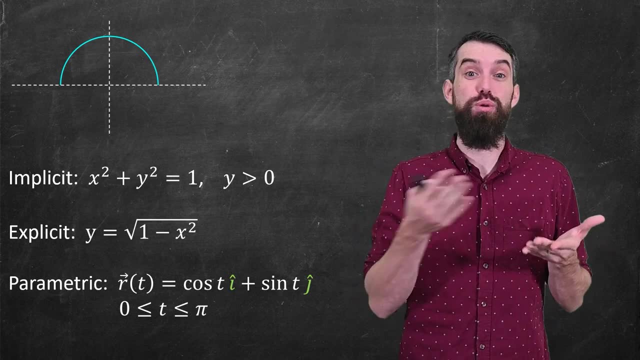 in this case sine of t, And whenever I come up with a parameterization I always have to specify the endpoints of my parameterization. So in this case I'm going only half of the circle, and so t is between zero and pi. So that was for this specific example of a half circle. If I'm going to be just 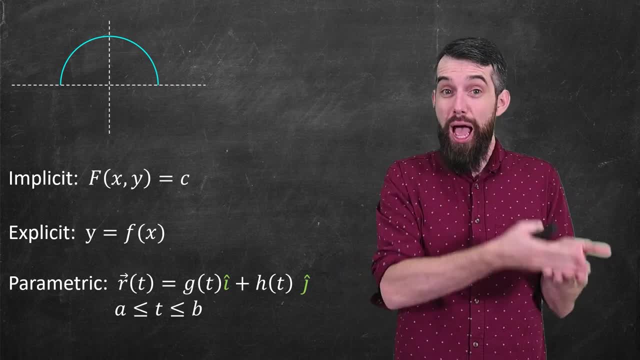 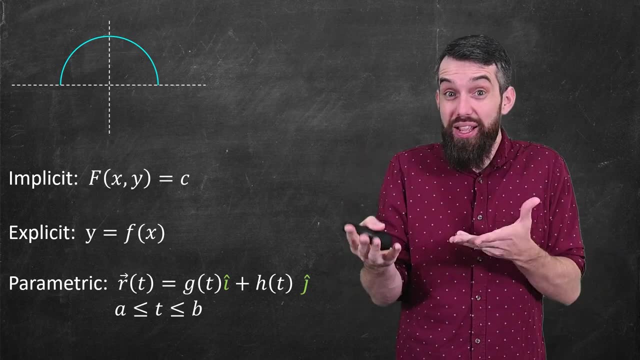 a bit more general. the implicit formula is just some function, capital F of x and y equal to a constant. The explicit is when I can solve it so that y is equal to some function lowercase f of x. And then the generic parameterization is just some position. 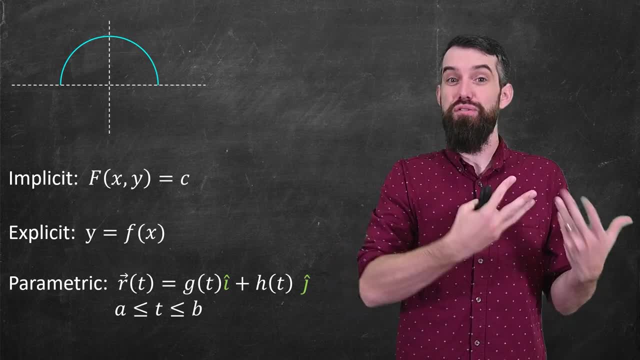 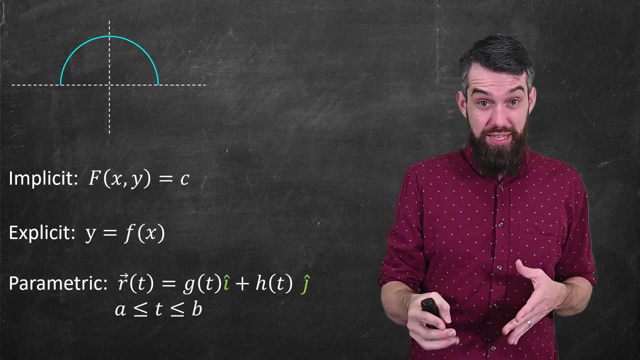 function r of t, which is just a function of g of t in the i-hat, a function h of t in the j-hat, and t bounded between a and b. Okay, so let's use that base for trying to now study surfaces. 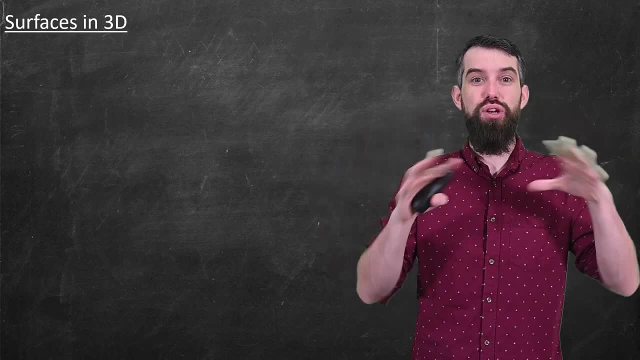 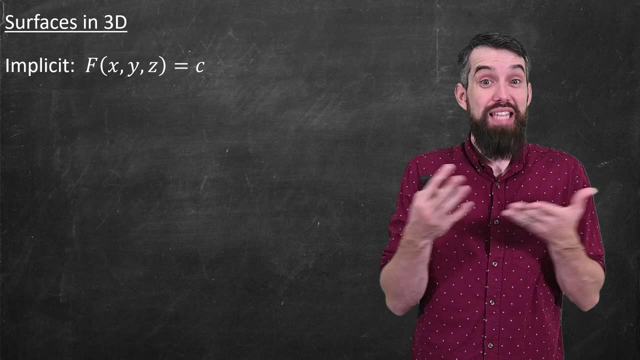 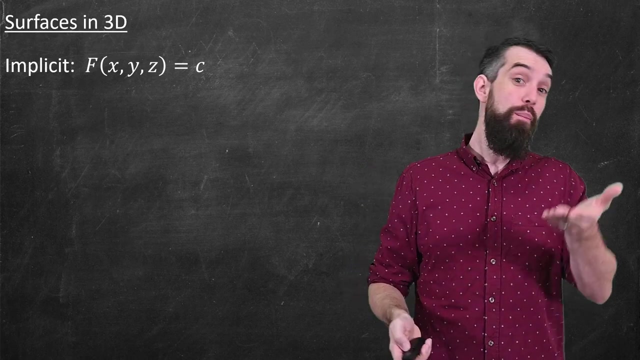 in three dimension. So I'm thinking about a two-dimensional object embedded in three dimensions. So it could be the case that I have an implicit description of this. That would be the exact same type of thing we've seen before. Capital F of x, y now and z is equal to a constant. It might 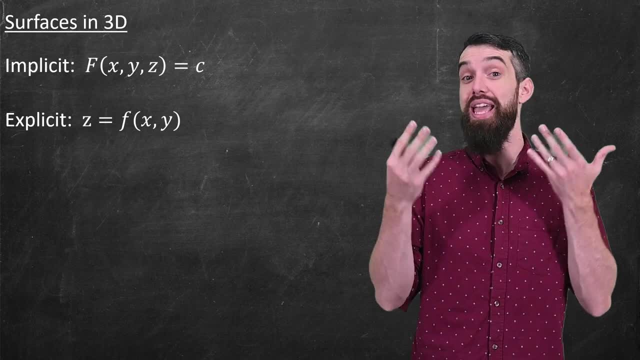 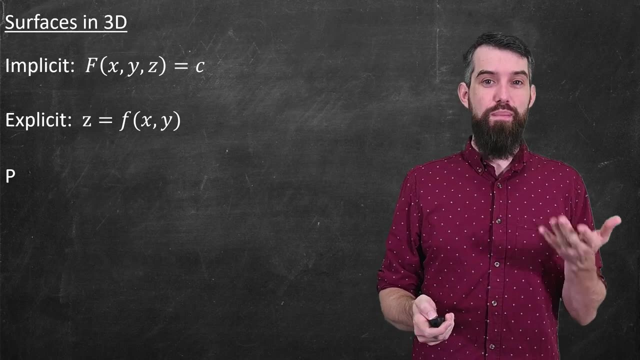 be that I could solve this for z. So z is given as a function of x and y explicitly. That sometimes could be the case and sometimes can't be. And then, most importantly, is the parametric formula. Now I'm going to have two parameters, So I'm thinking of surfaces as a two-dimensional object. 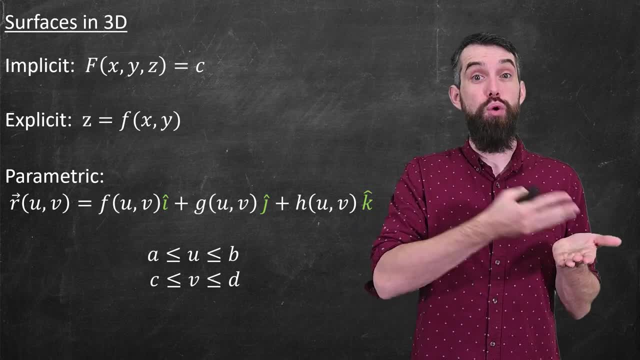 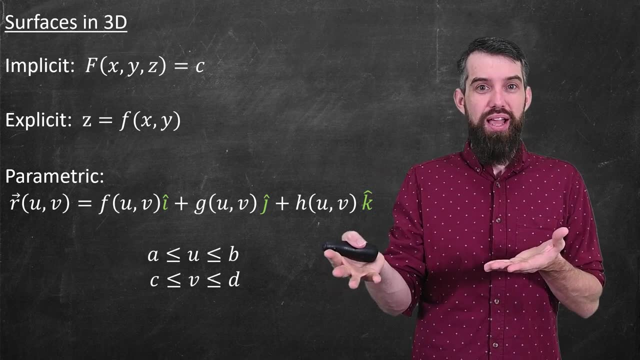 So there's two degrees of freedom, So I have two parameters and I'll call them u and v, And then, because it's living in three dimension, there's an i-hat, a j-hat and a k-hat component And each 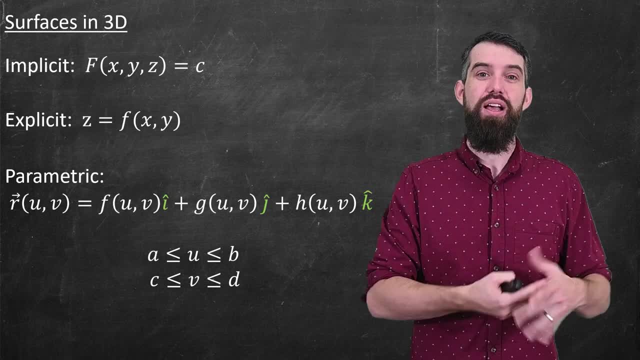 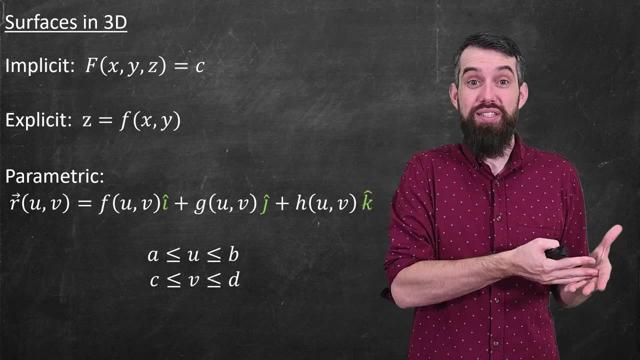 of those functions depend on the parameter. So it's an f of u and v in the i-hat, a g of u and v in the j-hat and an h of u and v in the k-hat, And then just the same as we've seen before. I have 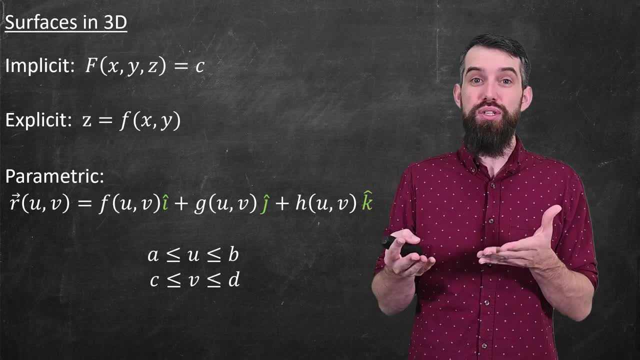 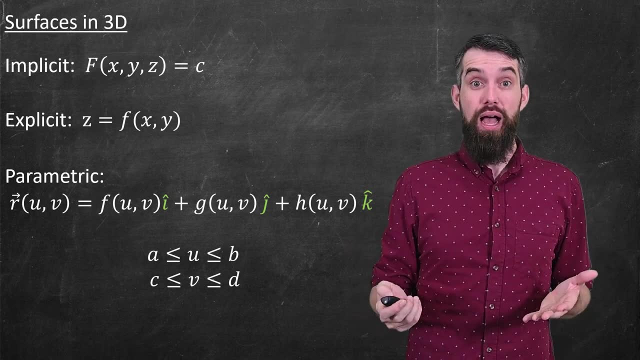 to say what are the limits of my u and my v. So u is going to generically go between an a and a b, and v is generically going to go between a c and a d. Okay, so let's see an example. I want to talk. 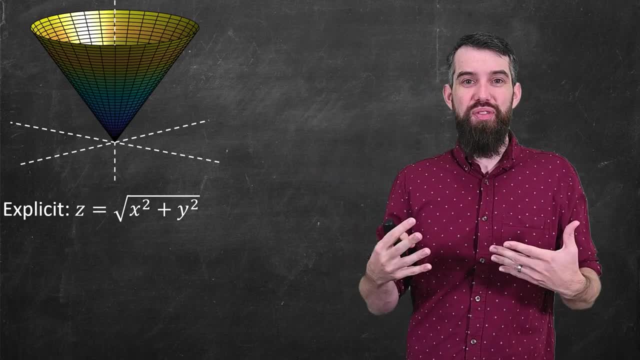 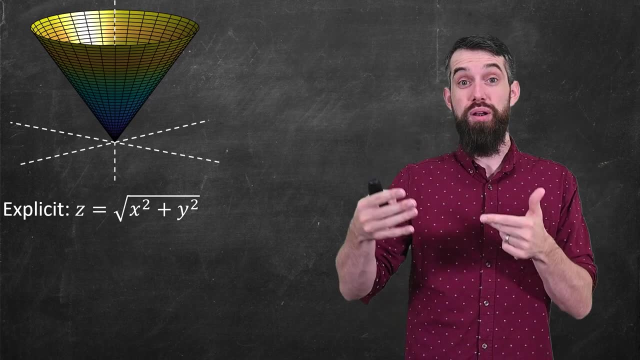 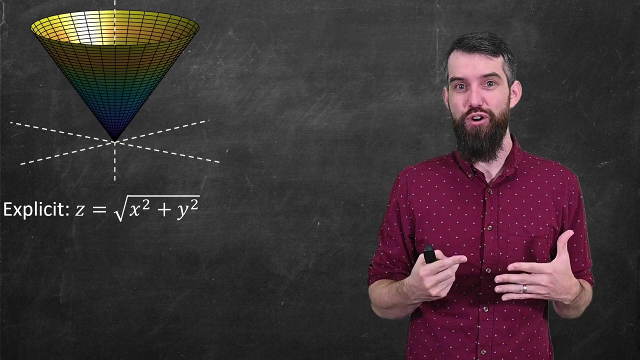 about the cone, that to think about this is just taking some line and rotating it around to make this cone, but I have an explicit formula for it: z is the square root of x squared plus y squared. Now, whenever you have an explicit formula, it's actually completely trivial to get an implicit formula as well. You. 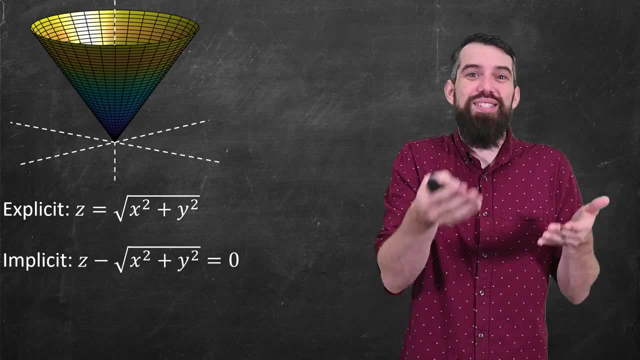 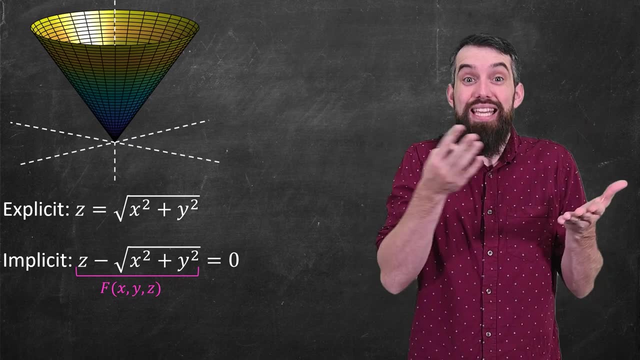 just subtract off. So the implicit is just: z minus square root of x squared plus y squared, equal to zero. We haven't done anything at all Here. the z minus square root of x plus y squared just is the capital f of x, y and z we've seen before. So the point is, if you have an explicit, you can always 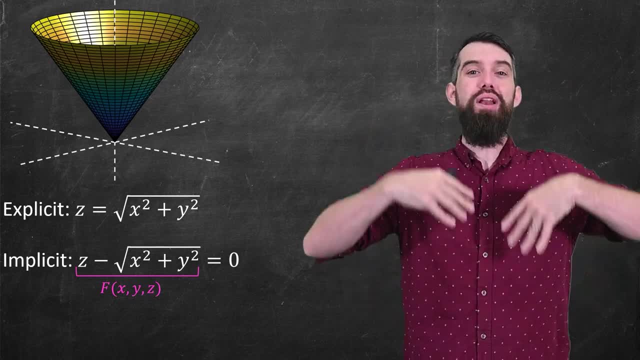 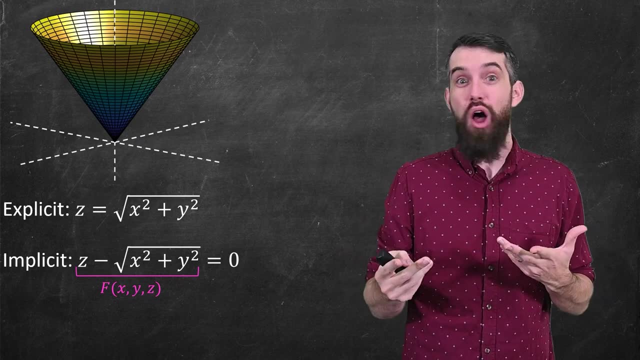 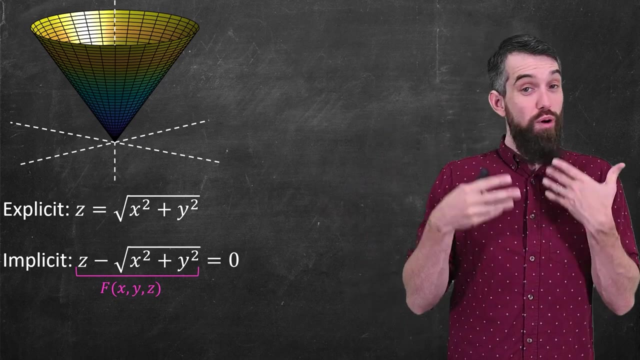 get to an implicit. If you start with an implicit, going reversing that process and trying to get an explicit is often just not possible. and even when it is possible theoretically, it's often not easy to do So. implicit to explicit is hard, but explicit to implicit is just trivial. So for the parametric. 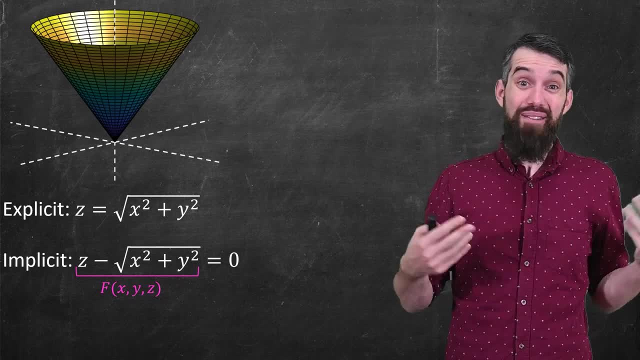 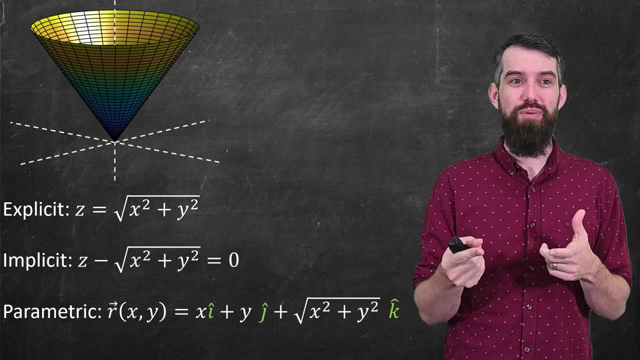 form. I need to come up with a choice for u and a choice for v. I have an x and a y already, so what if I just do that? Why don't if I set it to be the parametrization of x and y, in which case the x component is just? 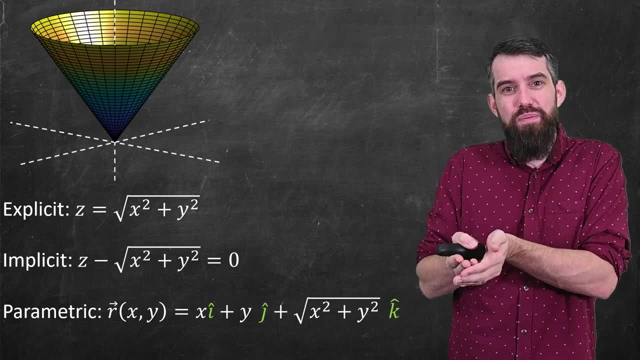 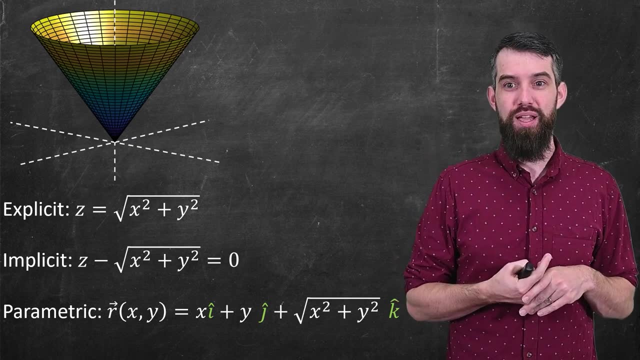 x. the y component is just y and then the z component because it's described as square root of x squared plus y squared. I just put in: square root of x squared plus y squared, k hat. So this is perfectly fine from the perspective of have you found a parametrization, but it's actually not that. 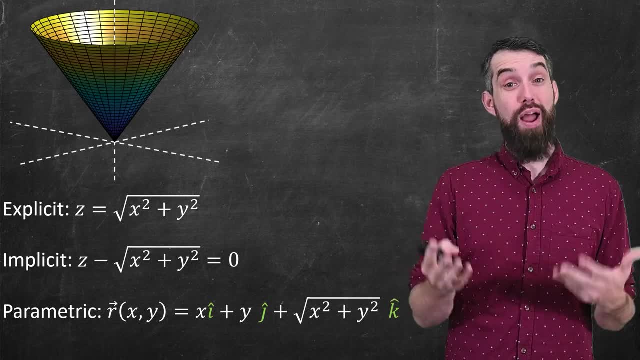 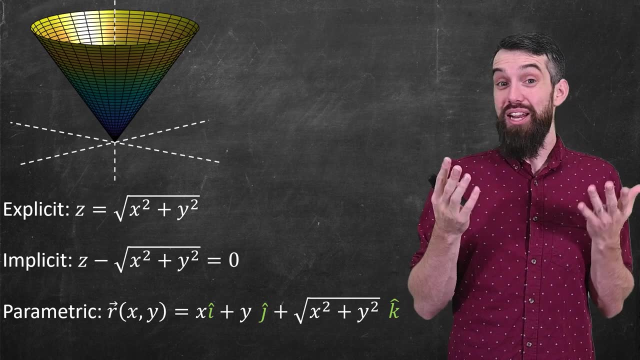 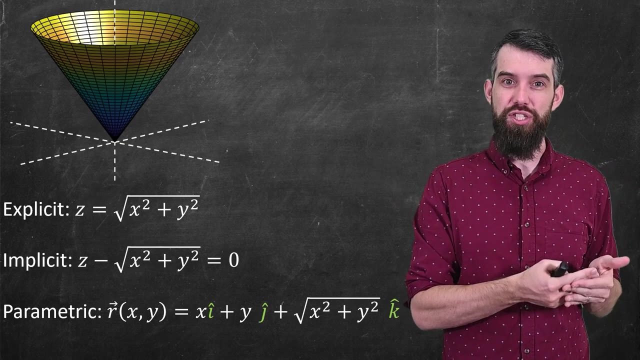 useful. What I really am going to want to do is come up with parametrizations that nicely capture the symmetries involved in whatever the surface was, and there is some symmetry. There's this sort of circular symmetry to a cone that is just sort of ignored by this choice of parametrization, and 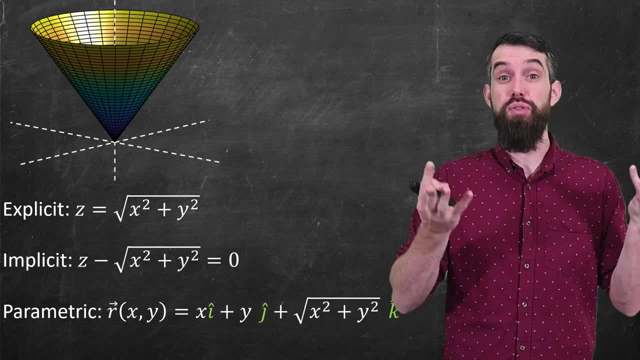 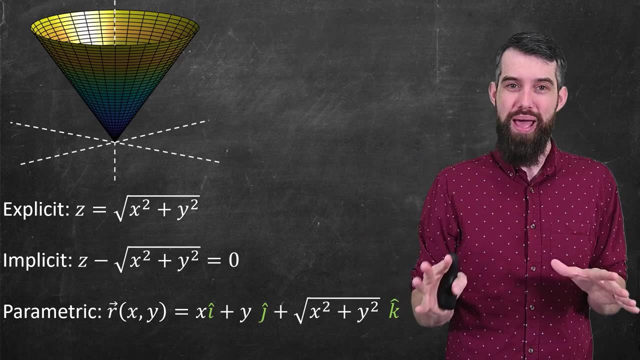 this is going to be a real problem for us later when we actually want to do things like compute the surface area of this and this parametrization is going to have some really messy square roots and integrals. It's going to be a whole mess. So I'm, in fact, going to get rid of the implicit. 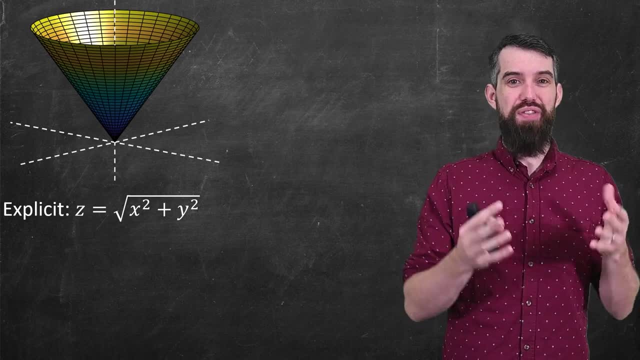 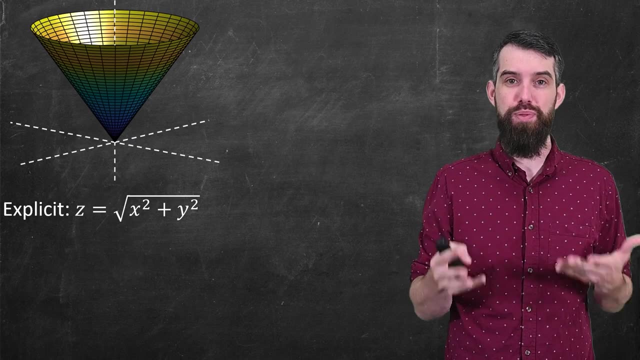 formula I had before because it was sort of trivial, and then I'll also get rid of that and then I'll get rid of the explicit formula. So this is a canonical parametrization that you could always do if you have an explicit formula. but might not be very helpful and we're going to 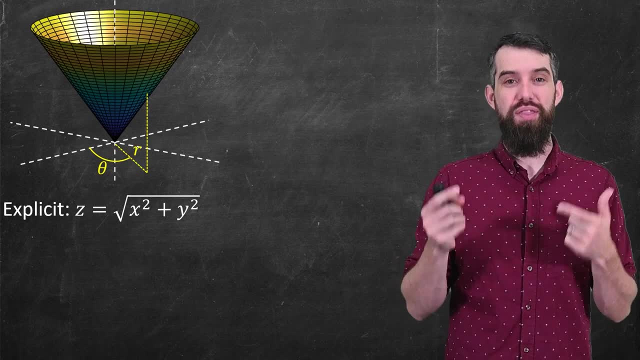 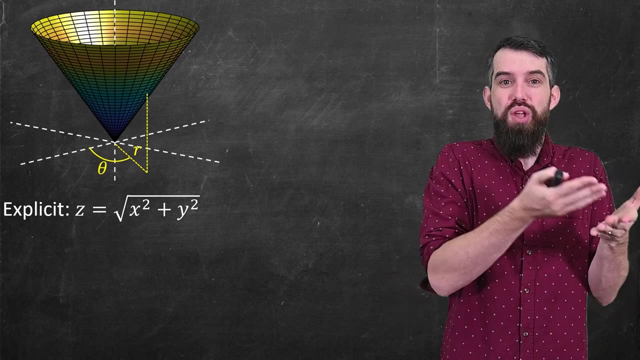 try to come up with a better one. So first thing, I'm going to put up a sort of cylindrical coordinates, if you will, on this picture. Basically what I do is I take a point on the cone and I project it down to the xy plane. Then I get some vector going from the origin out to the spot where it projects down. 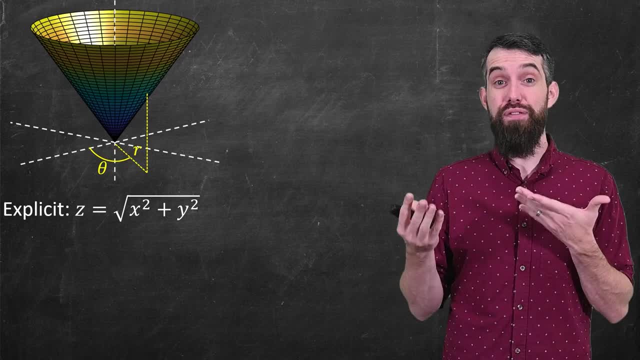 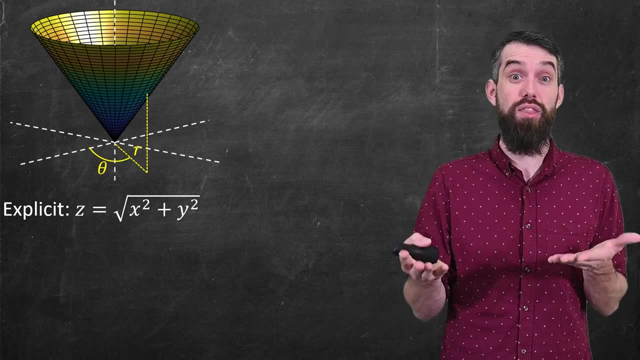 and that has a length of r, So r is defined to be that particular length. Then there's also an angle of theta that starts at the positive x-axis and rotates counterclockwise until it hits that line, the line we've labeled of having length r, Because my explicit formula was z equal to square root of. 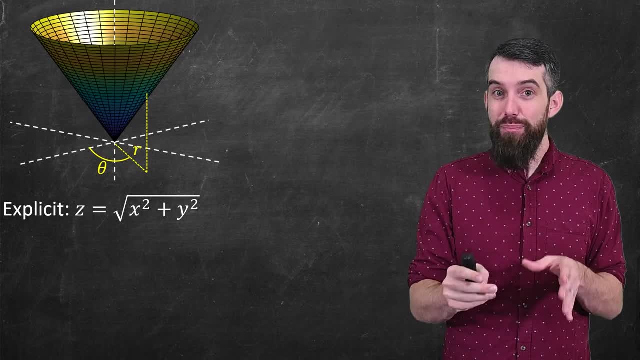 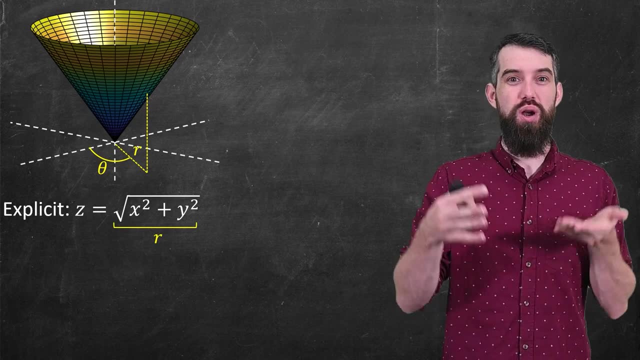 x squared plus y squared could have been anything. that's what I've chosen. this happens to be the exact same thing as r. r is defined, when you're talking about polar coordinates, as the square root of x squared plus y squared, This is just r. So the point is, if you know the theta and you know the r, 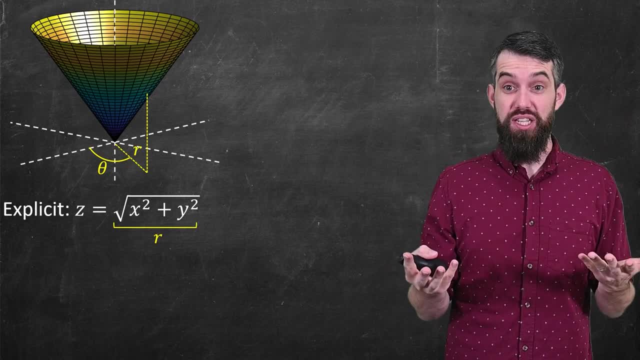 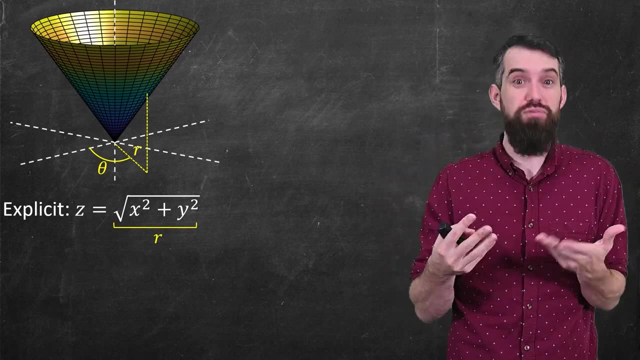 value. you know exactly where you are on the surface, because theta and the r is enough to describe a point down in the plane. And then, if you want to know how high up you should be, what the z value is, well, whatever your r was, that's what the height is as well. z is equal to r, And 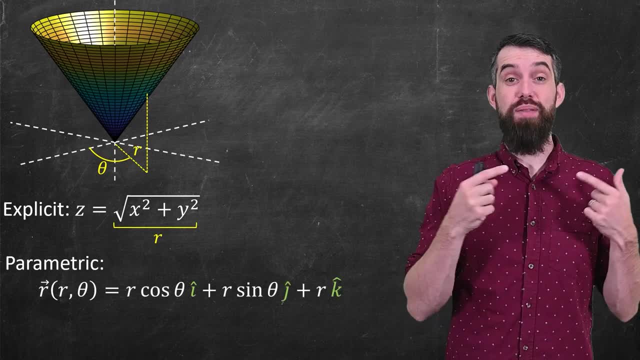 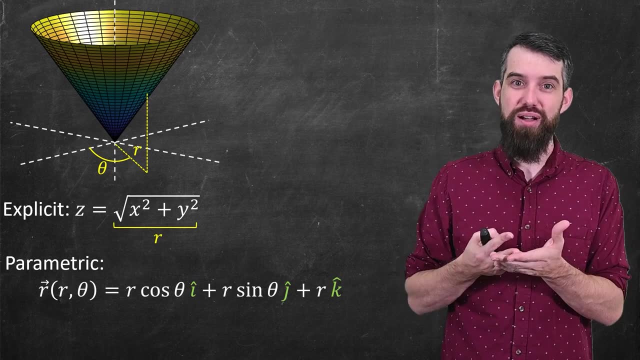 so we only need a theta and an r and as a result I can say: my parameterization is the position vector, r vector. There's two r's here, one with a vector hat and one without. So the position vector is a function of the two parameters of the vector hat and one without. So the position vector is a function of the two parameters. 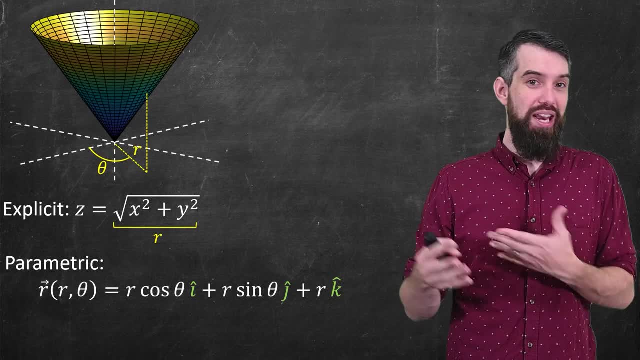 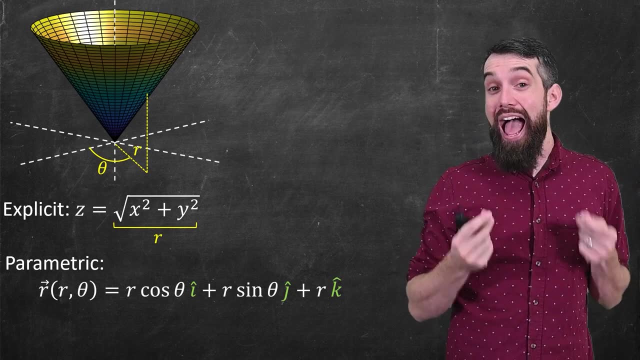 r and theta. And well, we do exactly what we've done any number of times. we've talked about polar coordinates in the past. We've gone and said: well, the i-hat is r cosine, the j-hat is r sine, but what we're adding now is the k-hat component, which is the height, which would normally be z. 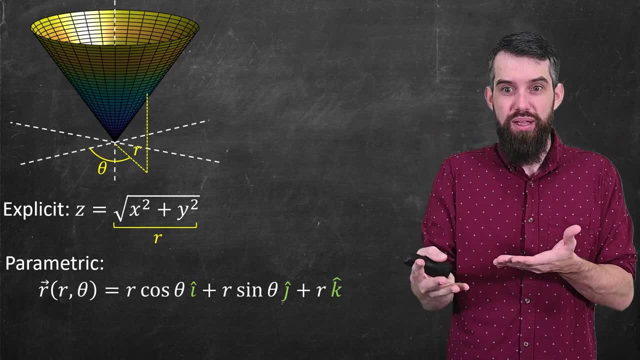 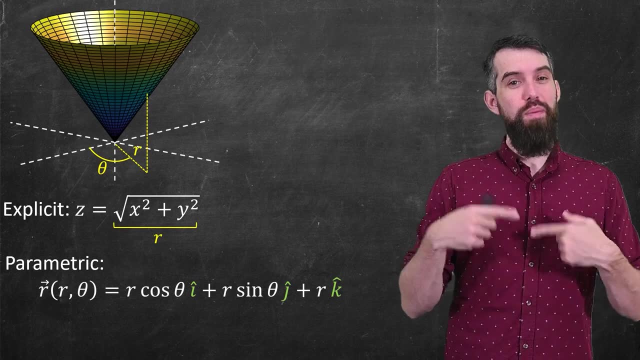 but since z is equal to r, it's plus r k-hat, And so if you know the r and the theta, we can describe where you are on this cone. Note that this is in slight contrast to what we might have done when playing with cylindrical coordinates in the past, where we would have had a. 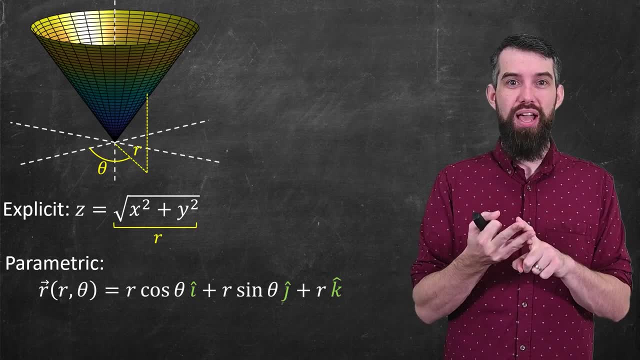 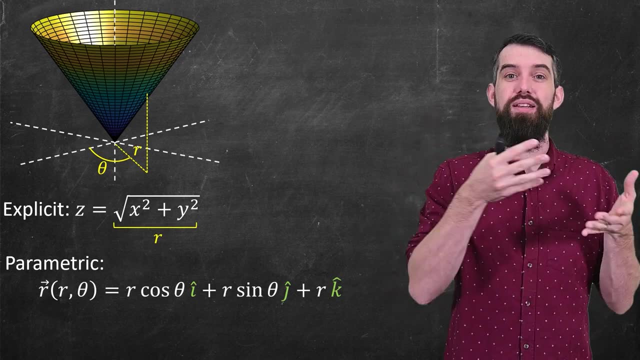 theta and an r and a z, all three of them floating around, and we would have had a triple integral that used all three of those variables. if we were computing, say, the volume of a region in cylindrical coordinates, That is three-dimensional. here we're trying to describe a two-dimensional. 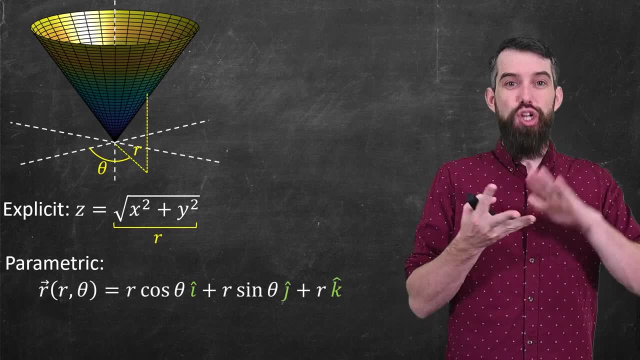 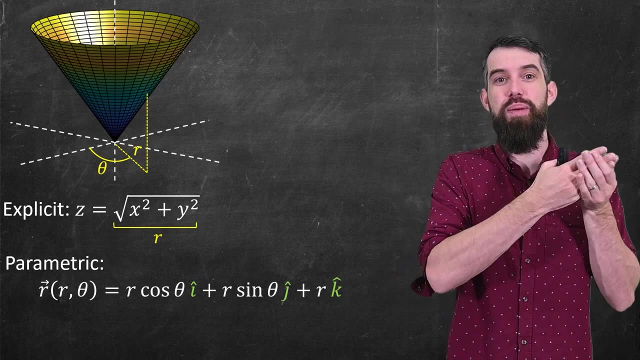 surface. and so, basically, what you do is you're choosing two of the three dimensions, r and theta, which is enough to describe everything, because we have that hook, that relationship, that z was equal to r, And so a third variable is equal to r and theta. So that's the three-dimensional. 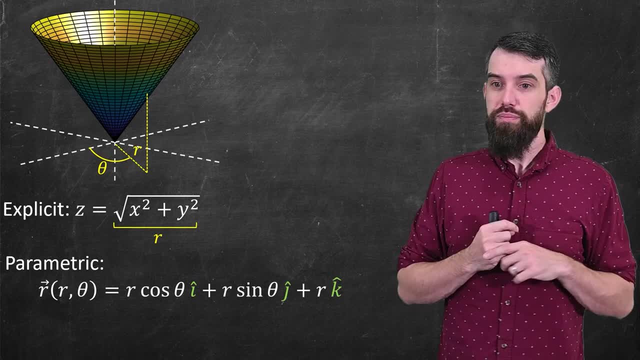 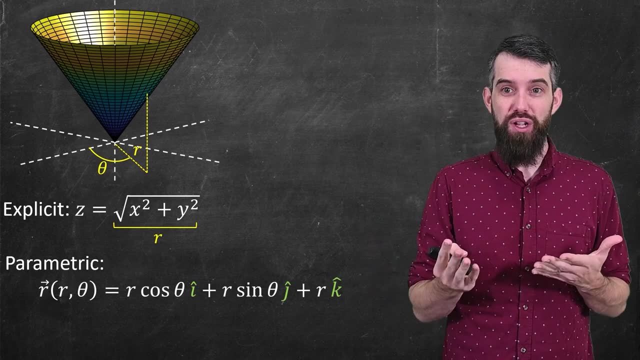 it needed to describe this here. Theta and r is enough. Now I have to be careful here, because I've been a little bit coy with you thus far. I said it's a cone, but which specific cone, Because what is the height of that top off, where it stops graphing it? I actually told it to stop graphing. 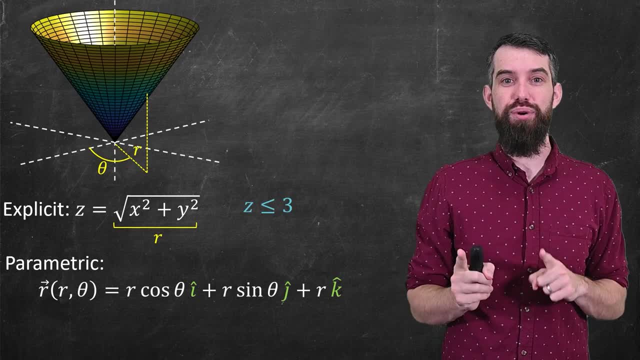 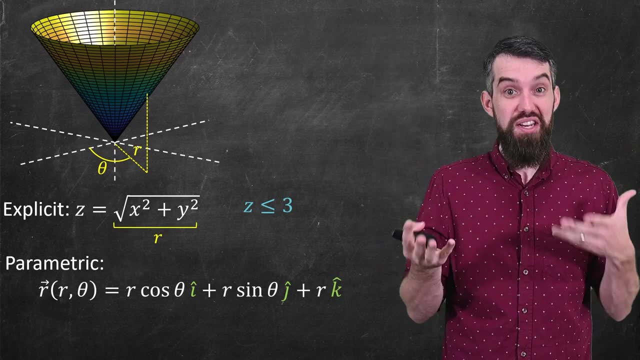 at z less than or equal to 3. so I'm going to put that out there: z is less than equal to 3 is a restriction on my formula, so it's only that portion of the infinite cone that it would be if you didn't have the restriction. Okay, so how does this translate into r values and theta values? and? 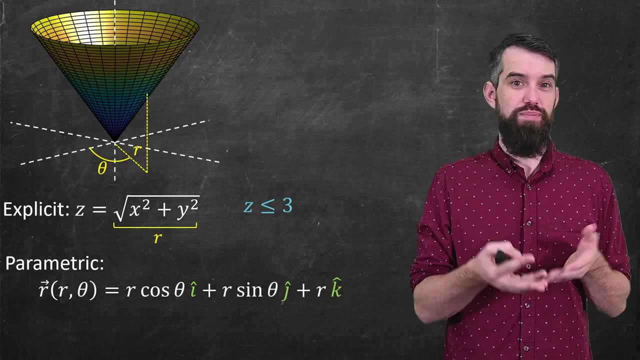 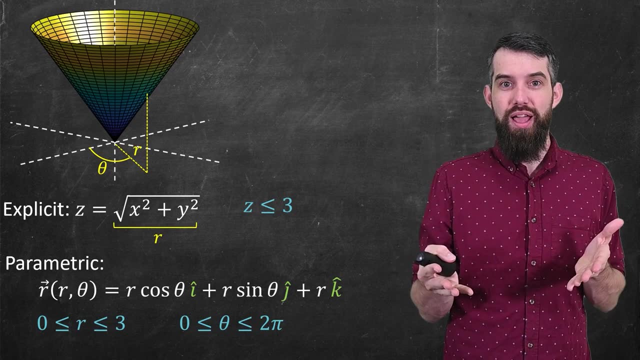 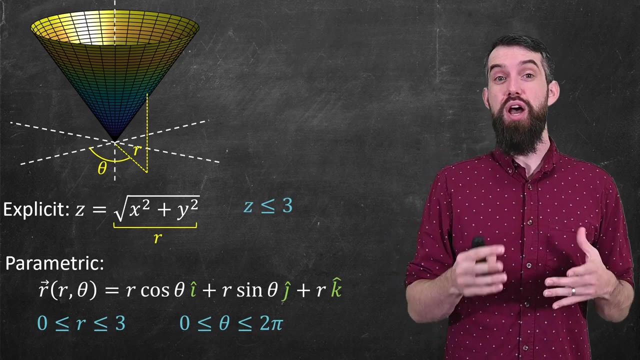 the restrictions on those. Well, z is equal to r. z is clearly positive here. it's a positive square root, and so what we have is that r is between 0 and 3 as well, And then theta is one revolution around, it's the entire revolution. so theta is between 0 and 2 pi, And indeed, whenever we try, 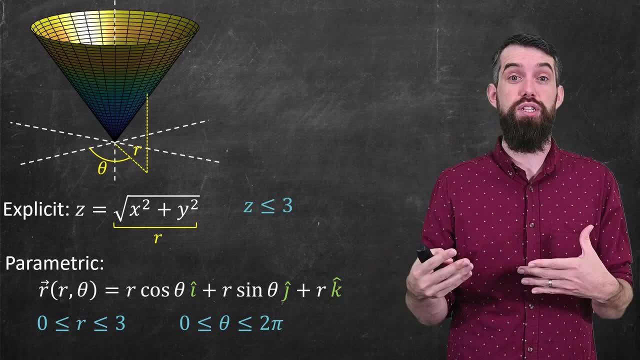 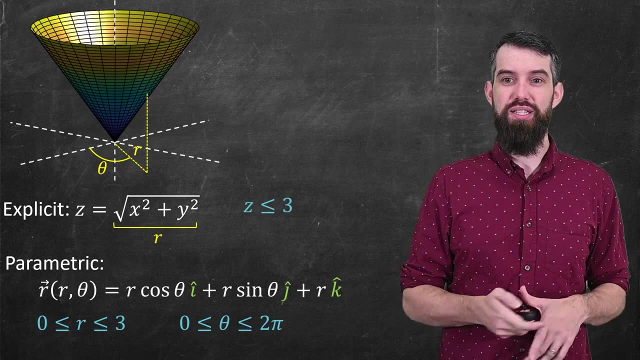 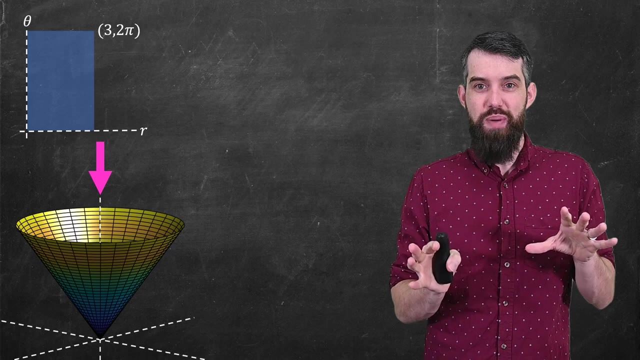 to write out a parameterization. we additionally want to describe the boundaries on the parameters, in this case on the r-value. The final way I'm going to think about this is: okay, let me just look at my cone. I want to imagine this as some sort of transformation. There is a two-dimensional space that has axes r and. 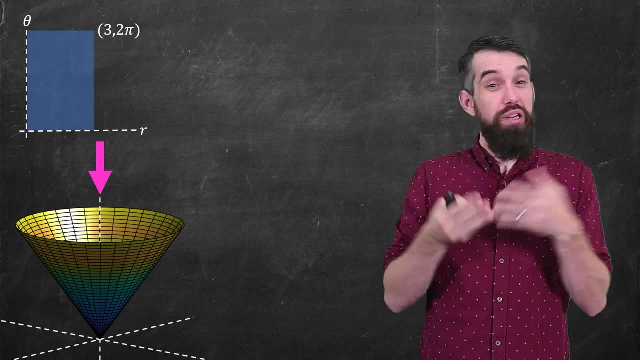 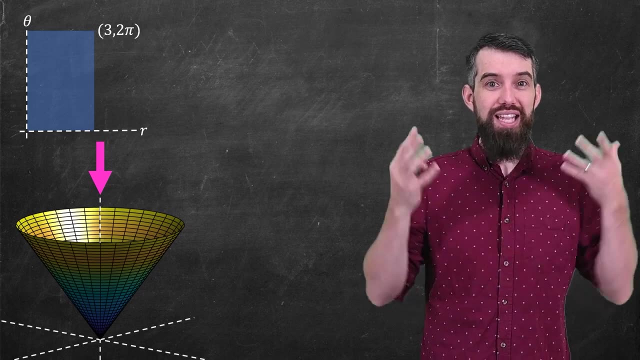 theta and in that r- theta coordinate system the region is very simple. It's just a rectangle on the r values going between the 0 and the 3 and the theta value between the 0 and the 2 pi. It's a simple region in that coordinate system. And then what a parameterization really is is a. 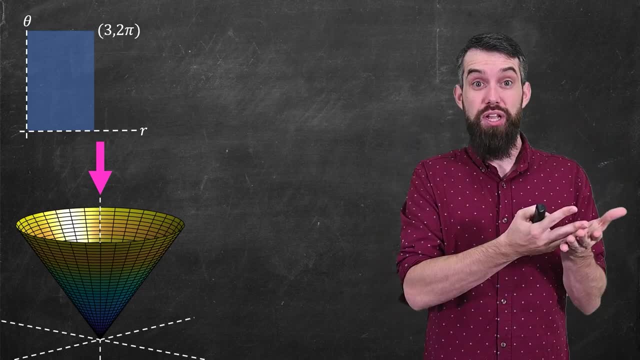 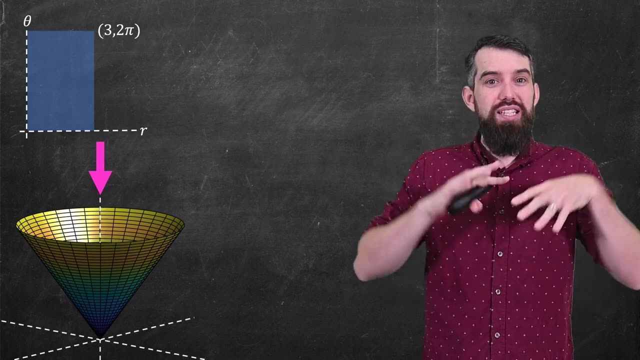 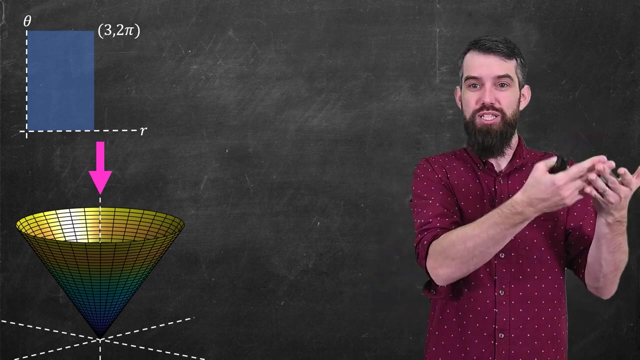 transformation from the simple region that I have, the r-theta two-dimensional region, to this more complicated two-dimensional region that is the cone embedded in three dimensions. The parameterization is just a way to map between this simple space and the r-theta plane to this more complicated. 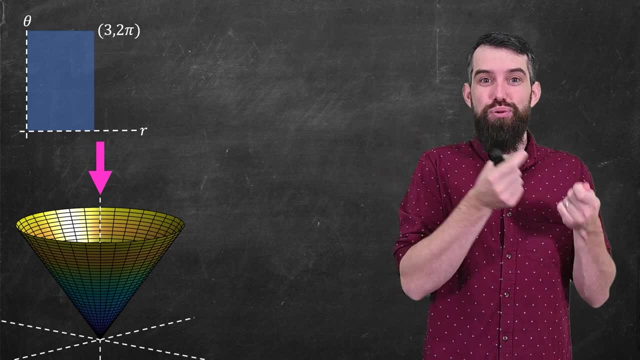 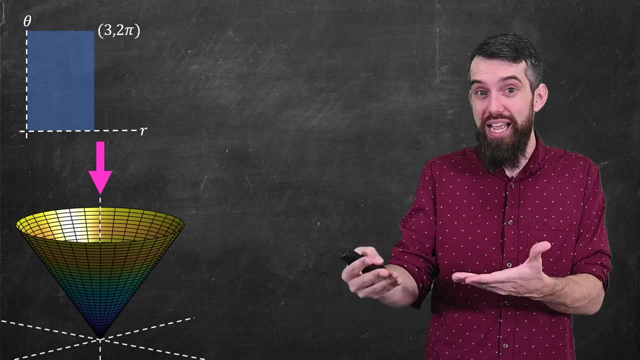 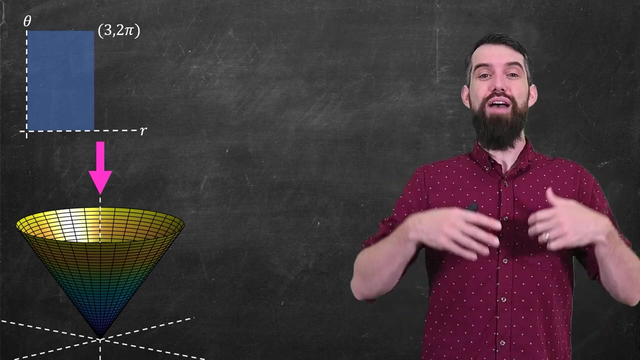 situation And because I've chosen natural parameters that reflect the underlying geometry, we're able to really simplify the process, and we'll see how that works in a little more detail coming up in future videos. So for now, if you enjoyed the video, please do give it a like If you have any questions about. 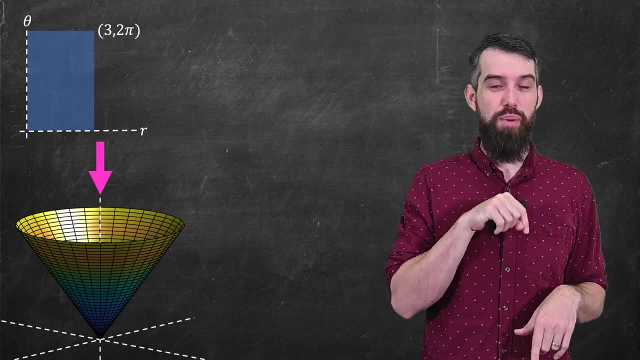 this video. please leave them down in the comments below. I try to get to as many questions as I possibly can and we'll do some more math in the next video.